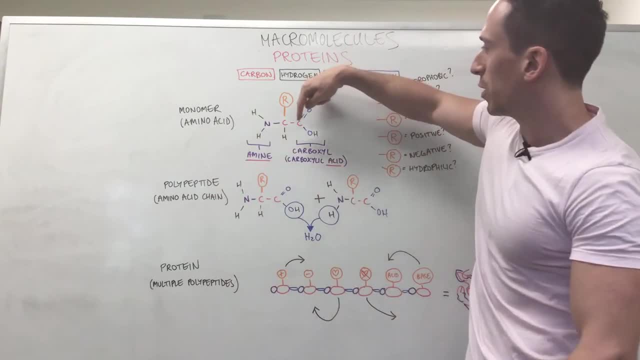 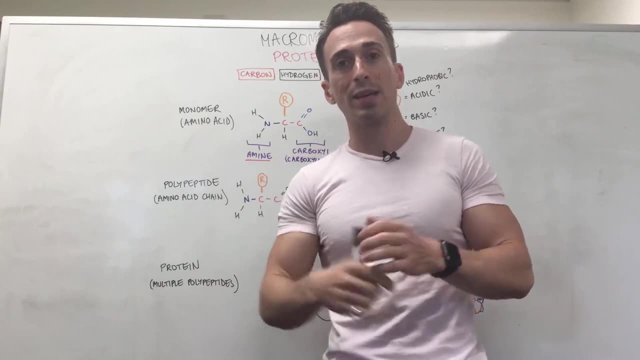 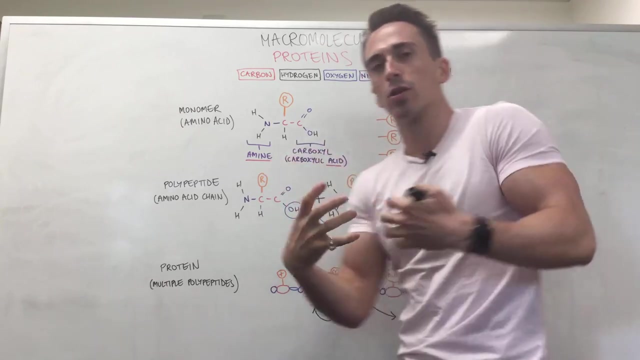 That's what's called an amine. Then what we've got is, on the other end, a carbon with a double bond, oxygen and an OH. This is called a carboxyl group. You would have seen the carboxyl group again in the fats and also in the carbohydrates, And together what you'll find is carboxyl is also. 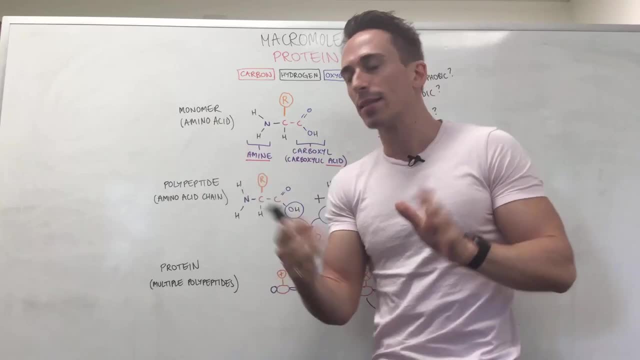 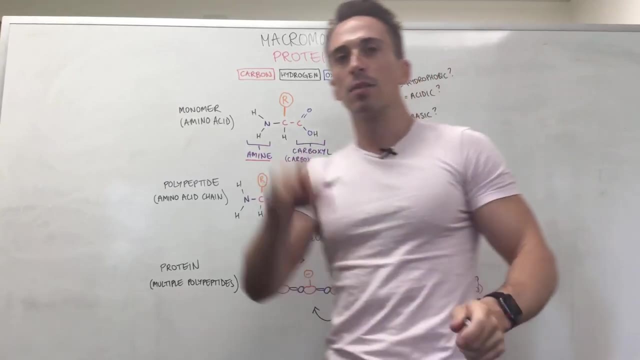 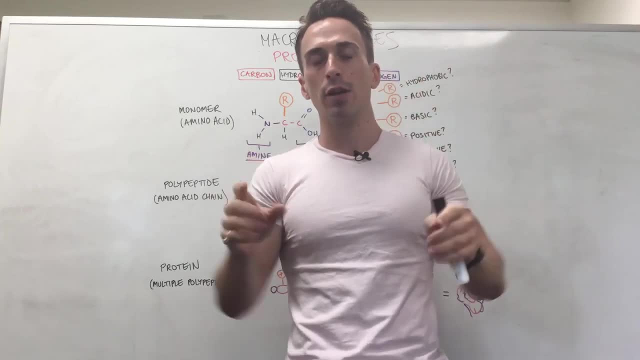 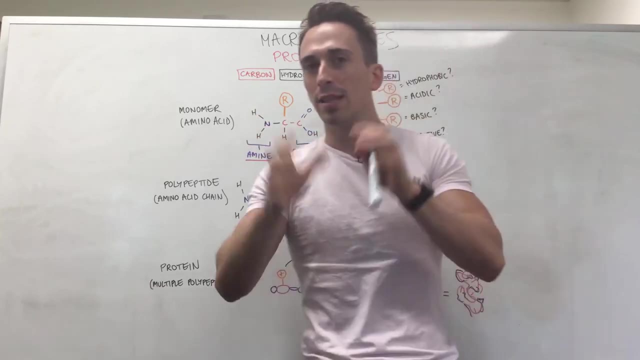 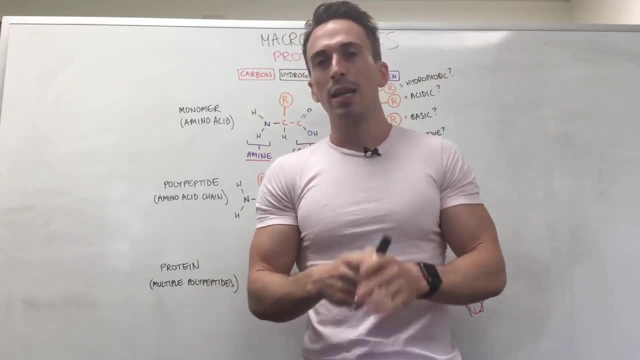 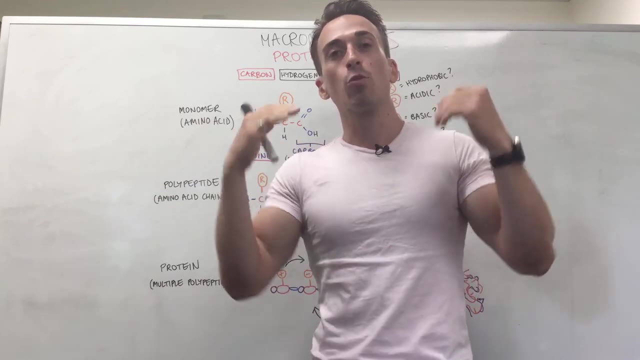 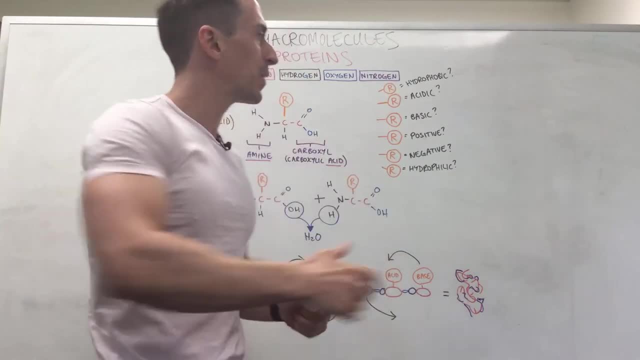 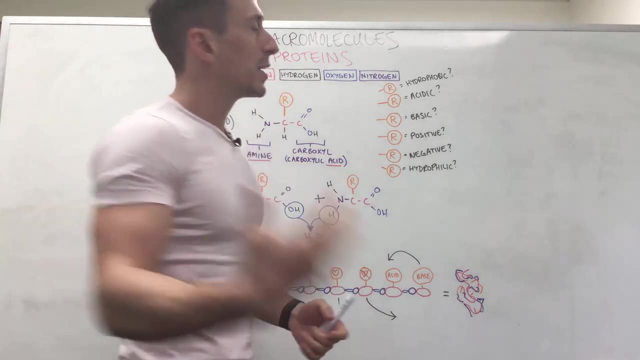 This functional group on the end. this is the thing, like I said, that makes them different. Some of these functional groups have specific characteristics or properties or personalities that make them so different. For example, some may be hydrophobic. That means they don't like. 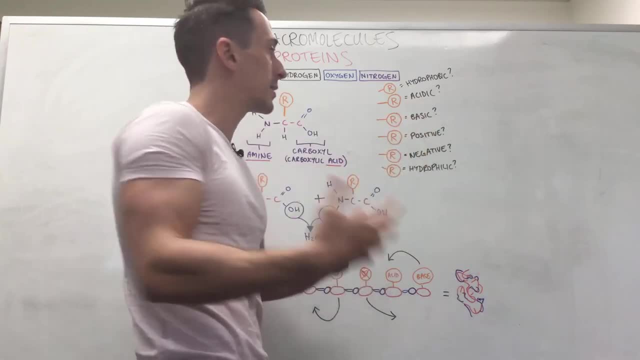 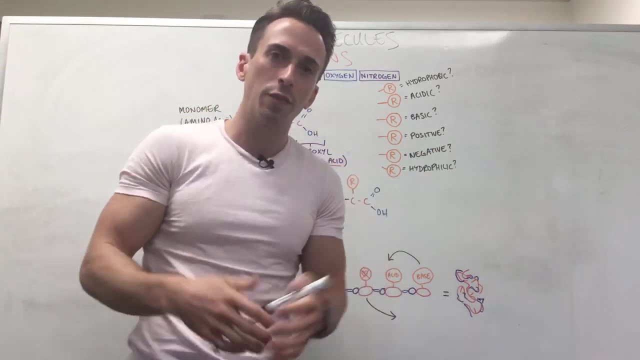 being near water. Some may be acidic, Some may be basic, Some may be quite positive, Some may be negative And some may actually like water being close to water, called hydrophilic. Now, this is important because when we take an amino acid and we click it together with another amino acid, 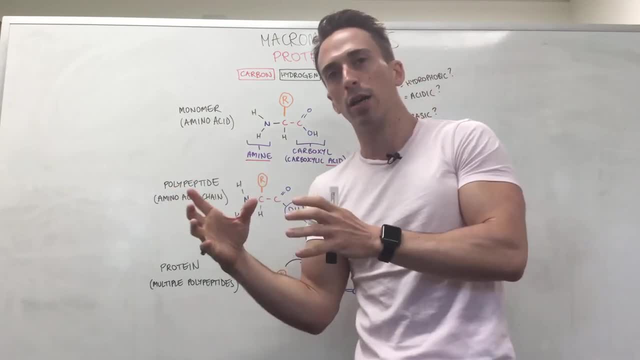 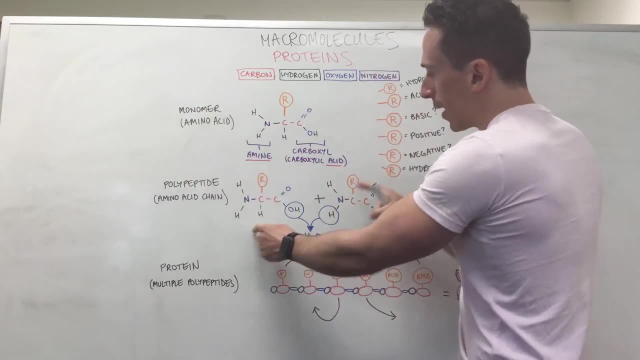 which is what we're doing here. we're starting to create what we call a polypeptide. this is a polymer, this is a chain of amino acids. so we simply take one amino acid and another amino acid and, just like we spoke about when we're clicking together monomers of carbohydrates like glycerol for 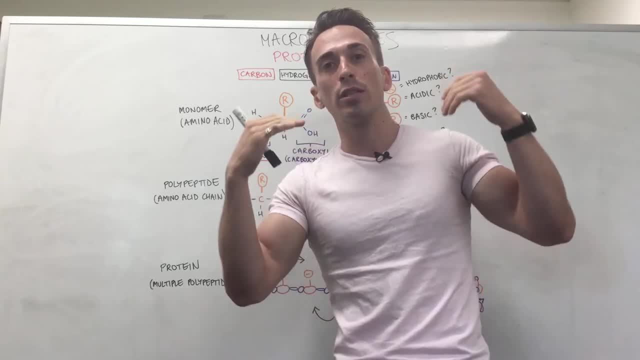 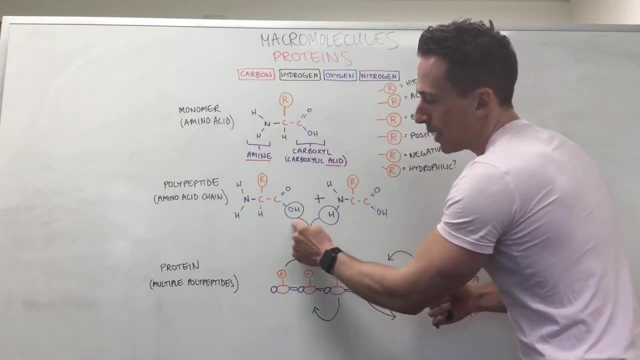 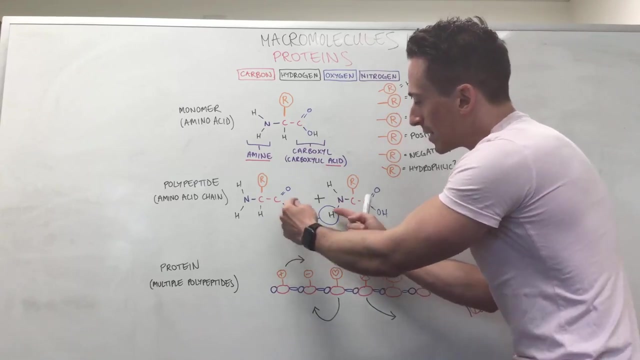 example, and when we're clicking together fats we go through a process of dehydration. we need to remove a water molecule and here you can see, we take the OH group here from the carboxyl end of one amino acid and we take a hydrogen from the amine side of another amino acid. together we've 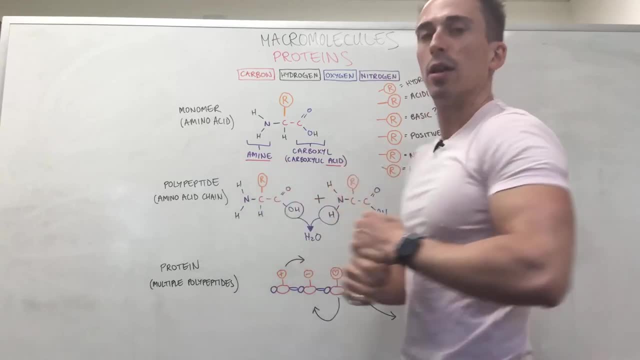 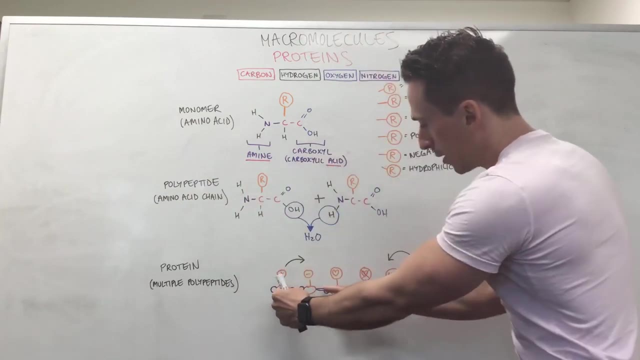 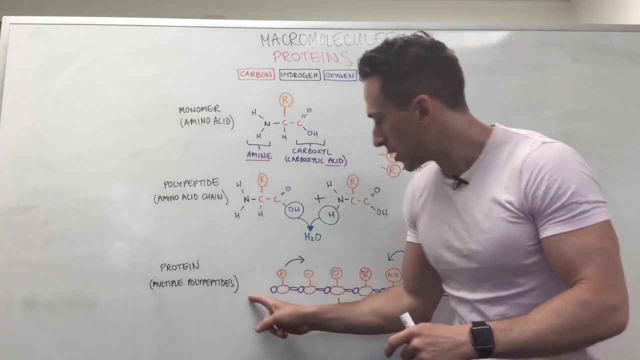 taken away: water, H2O, and now we've clicked two amino acids together and we continue to do this to create a polypeptide. now, when we create a nice long polypeptide chain, which we've got here, we're starting to move towards something that's resembling a protein, but not yet what you'll see. 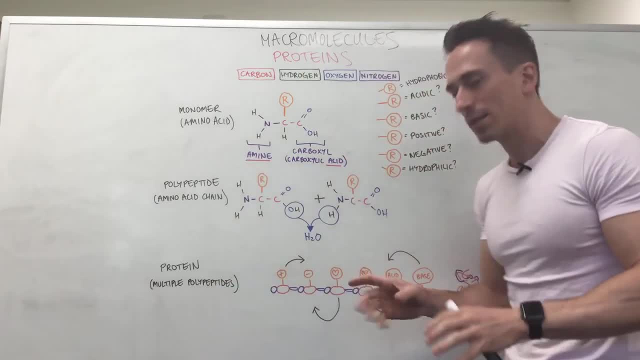 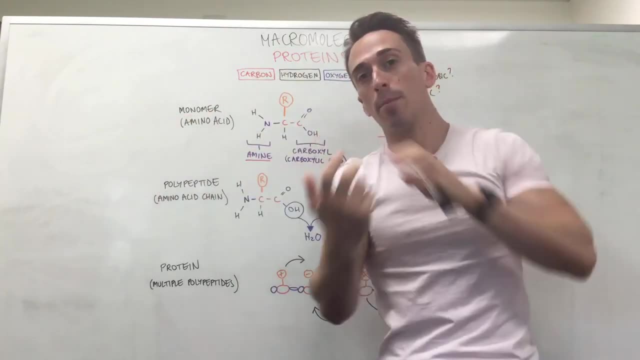 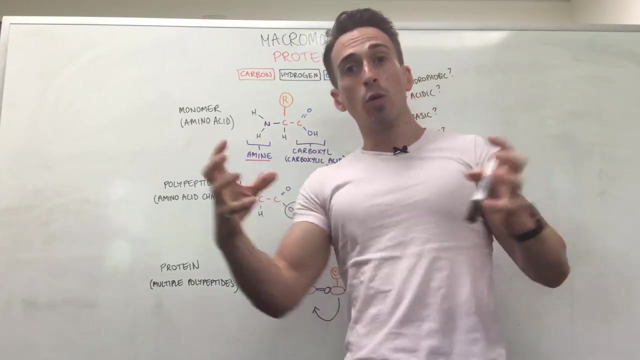 is. we've got this nice long chain with all these different functional groups. now it's the functional groups that are going to alter this nice long linear polypeptide and tell it to fold in upon itself. how does this work? okay, if one of these functional groups is positive and another is negative, they're going to 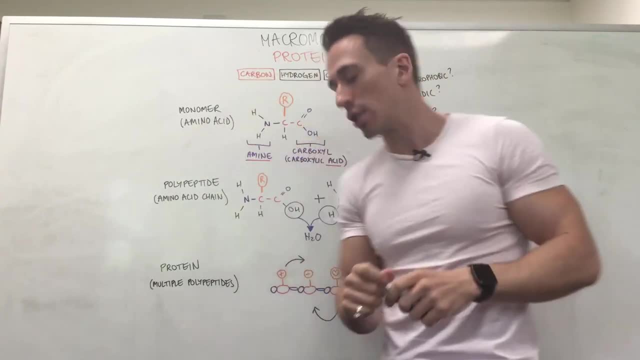 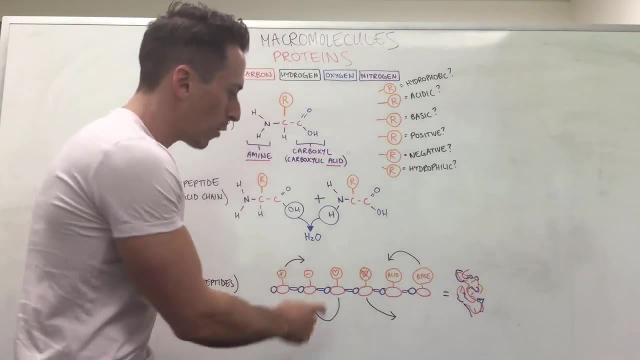 want to be close to each other. okay, so they arrange themselves to be near each other. if both are positive, then they'll want to be away from each other and they'll fold themselves so they are away from each other. you may have one that likes water or a couple that like water. that means they're 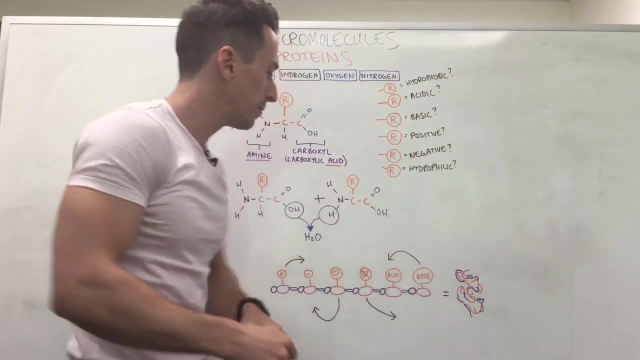 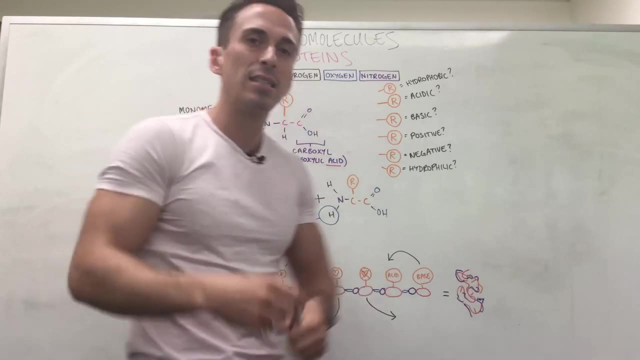 going to fold themselves so they're exposed to the liquid environment. you're going to have some that hate water so it wants to embed itself deep within the protein. you're going to some have some acids and some bases and this also is going to alter the way that it folds itself and what ultimately. 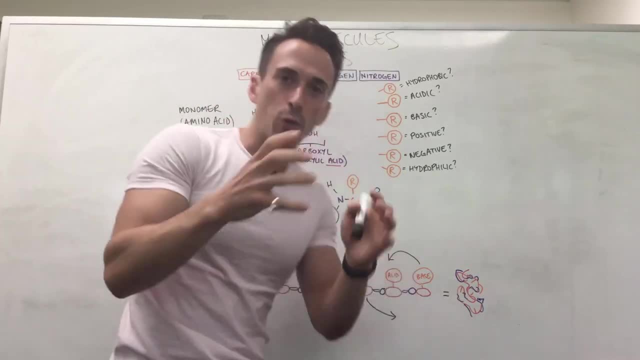 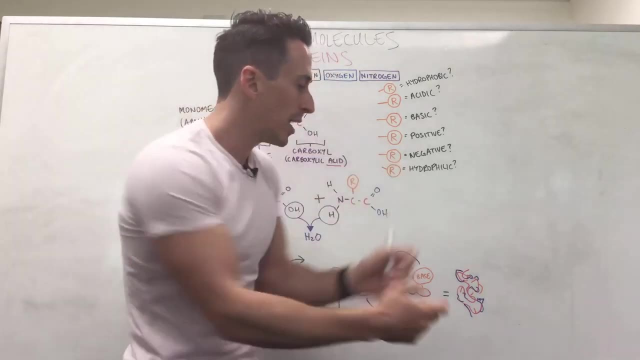 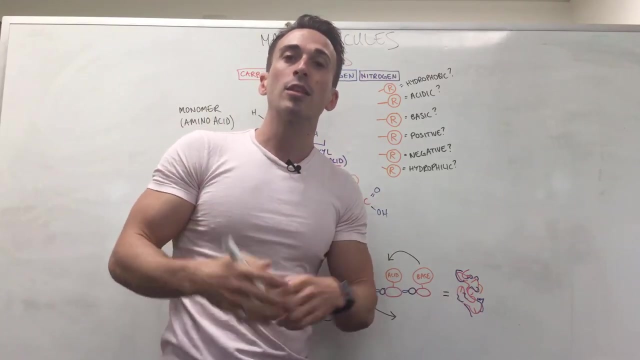 happens. it happens is you get this three-dimensional, what we call a quaternary structure of a folded polypeptide or group of polypeptides into something called a protein. and now this folded protein is what actually has the function in our body. there's around about 20,000. 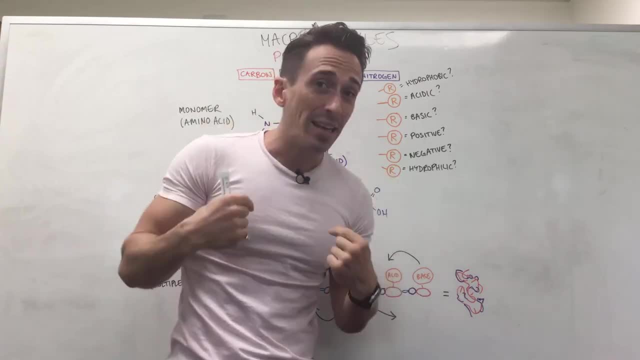 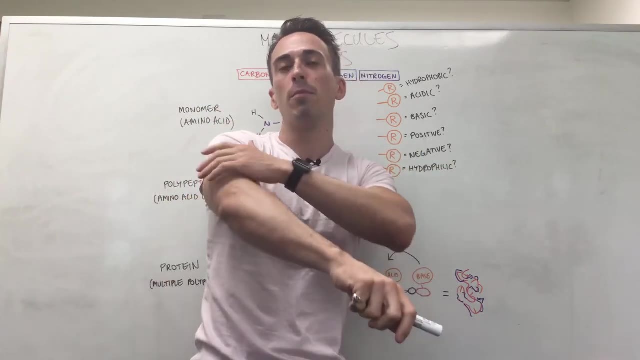 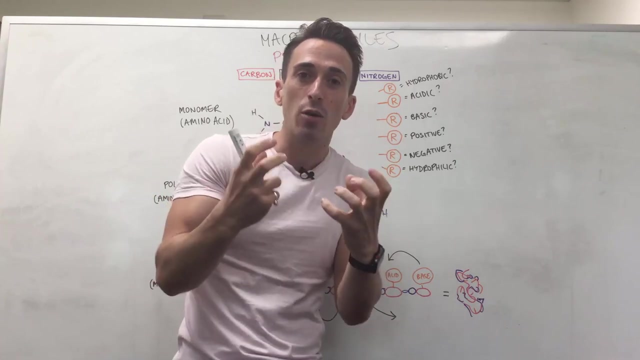 to 50,000 and proteins that our body makes, okay, from our genetic material. and when you're looking at me right now, you're basically looking at all my proteins, so it makes up the majority of my skin and my eyes. it has all the functions in the body, it. they basically make enzyme or they are enzymes. 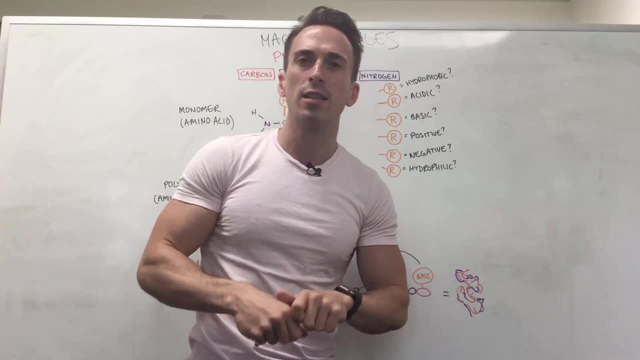 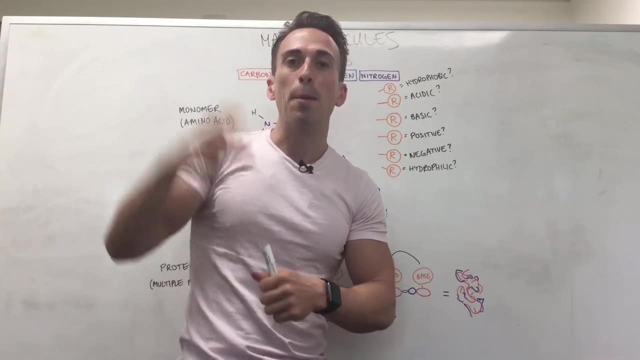 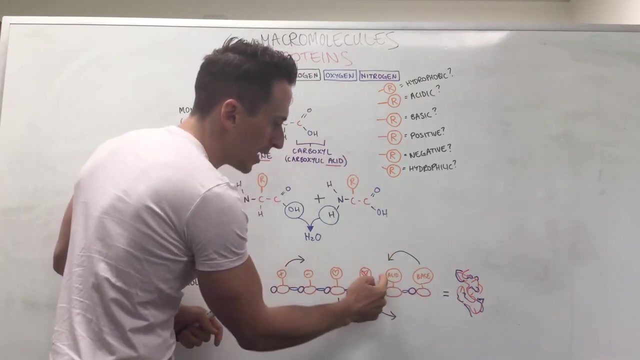 so this makes reactions happen millions of times faster than they would without enzymes. they shuttle things by picking things up and taking them elsewhere. they can be receptors. they can bind to other things. proteins have all the function in the body, so they're extremely important and it's these functional groups that fold it into its functional property. and if you have a problem,